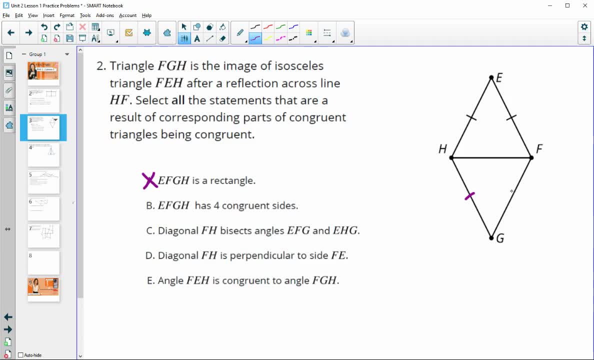 So GH and HE are corresponding parts, And FG and EF are. So these are going to be corresponding parts of congruent figures as well from flipping, So all four sides being congruent. The diagonal FH bisects the angle, and that would be true because this angle, here the corresponding angle, is here. 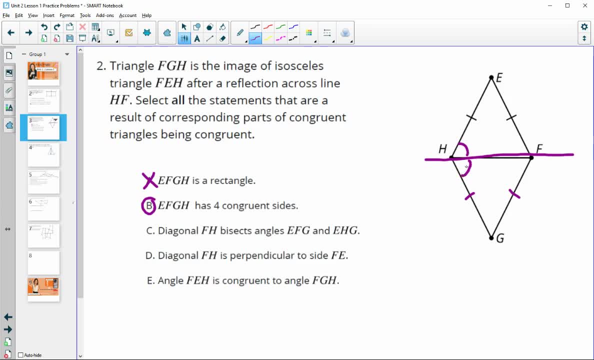 And so then those two angles are equal to each other, which then is the definition of bisector Diagonal FH is perpendicular to FE. Perpendicular means 90 degrees, And we don't have that Angle FEH, So FEH, this angle here is congruent to FGH. 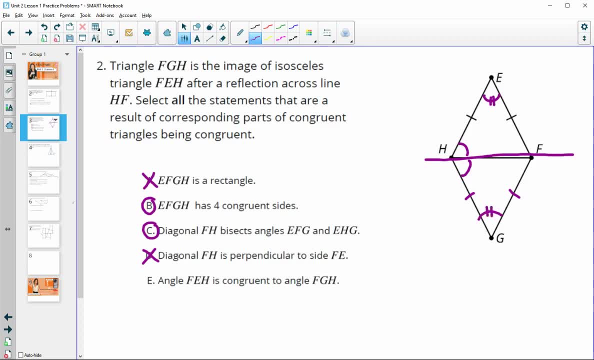 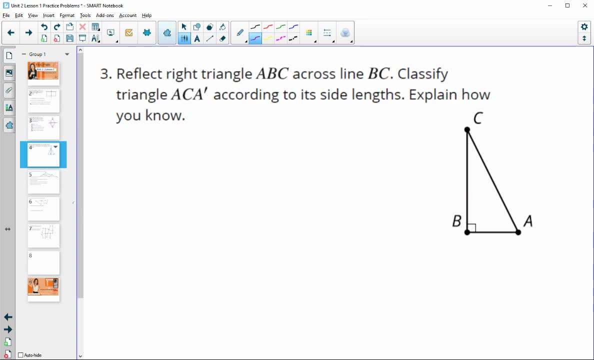 So this angle here and that would be true. Those are corresponding parts. Number three reflect triangle ABC across line BC. So let's do that, So we're going to reflect it, We're going to cross there And then let's label those parts. 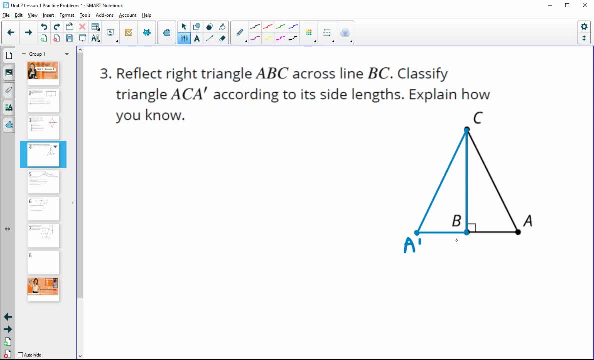 So A would reflect over here. So this would be A, prime, B and B. prime would be at the same point, And C and C prime would be at the same point According to its side lengths. explain, So classify the larger triangle. 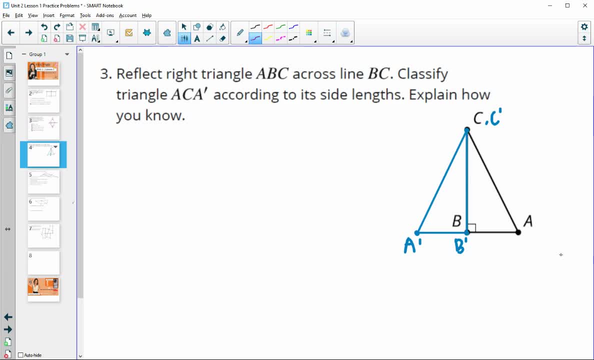 Okay, So we're going to classify triangle ACA prime, So let me draw that in here. So we're going to be looking at classifying this triangle And so we know that this side is equal to this side because of them being corresponding parts. 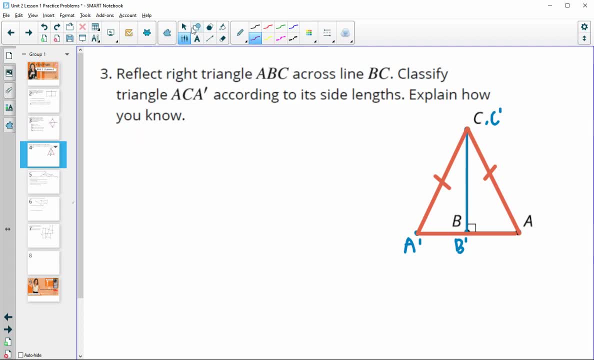 So we know that this is an isosceles triangle. So we know that this is an isosceles triangle Because AC and A prime C- A prime C- are congruent to each other since they are corresponding parts of the reflection. 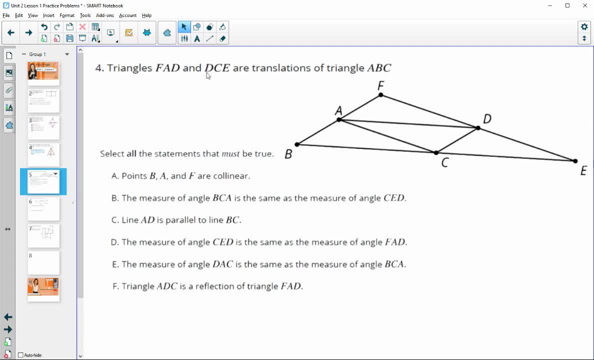 Number four triangles FAD And DEC are translations of ABC. So we see, this ABC is the original. If we slide it here it would land on DC, And if we slide it here it would land on FAD. So we know that those triangles are congruent to one another. 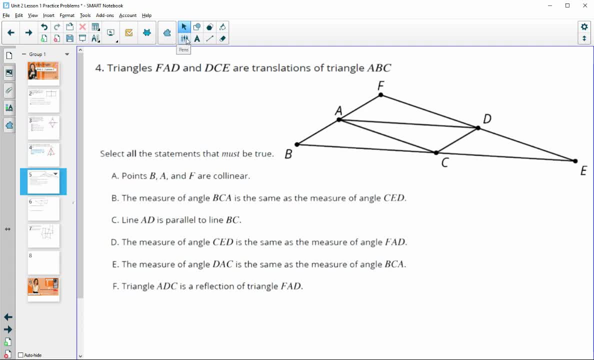 Select all of the statements. that must be true. So points A, B and F are collinear, And this is true, Because a translation would take a line parallel to itself or to the exact same line, So this line right here is actually going to be taken to itself. 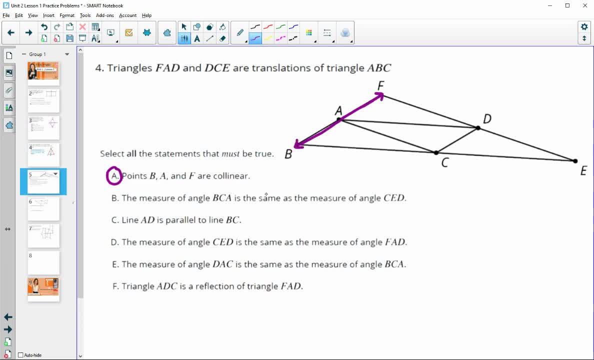 So then this will be a line, And so B, A and F are all on that line, meaning they're collinear. B, the measure of angle BCA. So this angle here is the same as the measure of angle CED. 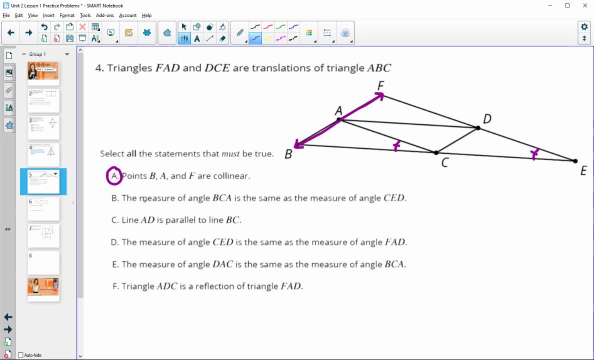 And that would be true, since they are corresponding Parts of those congruent triangles from the translation Line AD. So let's find AD here. So here's line AD is parallel to line BC And that will be true because of the translation. 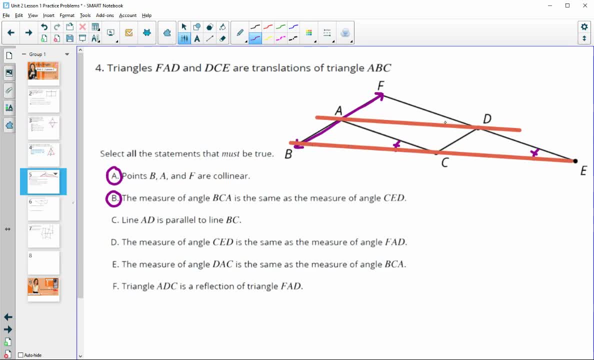 Again, BC, when we translate it up, goes to AD, And a translation will either take the line parallel to itself or to itself. So this one's taking It parallel, And so that would be true. The measure of CED is the same as the measure of FAD. 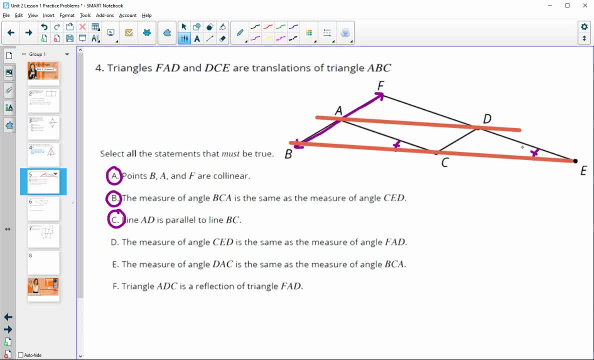 So CED is right here- Is the same as FAD, And that is not true. Those are not corresponding parts. Okay, This one would be the corresponding part with it: The measure of DA DA. So this one again. 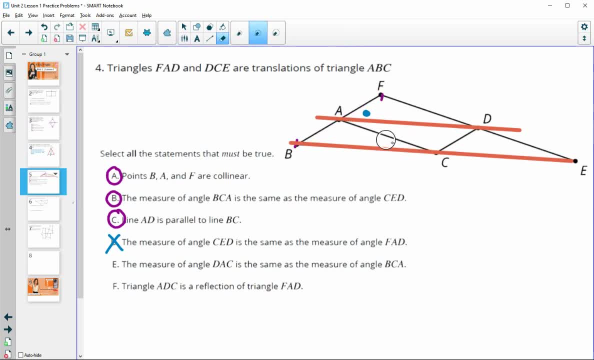 So let me get rid of some of this other stuff here. All right, The measure of DAC, which is actually this angle. So DAC is here And the measure of BCA are equal to each other, And this is going to be true because those are alternate interior. 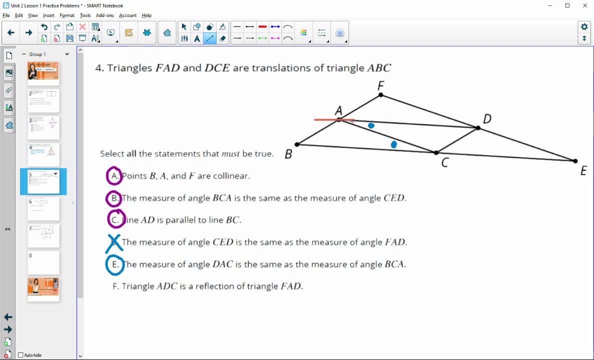 So if I put those lines back on there- Remember we said that AD is parallel to BC, And then AC would be the transversal And we end up with alternate interior angles there. So that's true. And then triangle ADC. 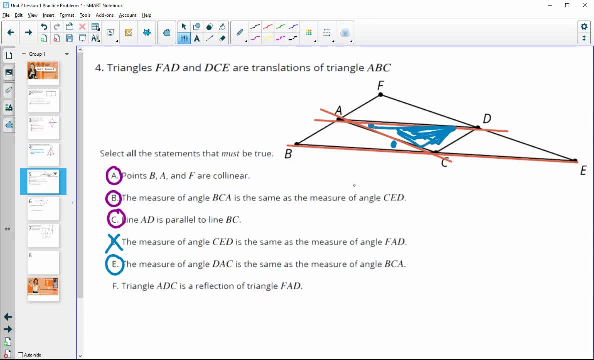 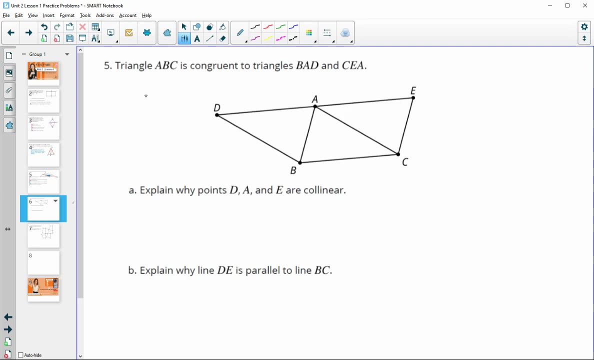 So this kind of middle triangle here is a reflection of FAD, And that is not true. If we reflected this point over, It would land more like here rather than here. So that is false. Number five ABC is congruent to. 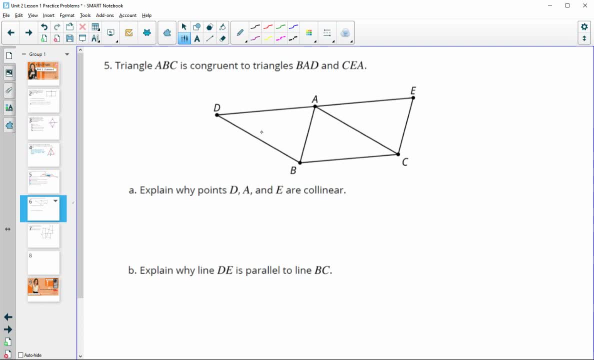 So ABC, this middle one, is congruent to BAD and CEA. Explain why points DA and E are collinear. So if we know we can kind of see these different angles. So I've got this angle here. 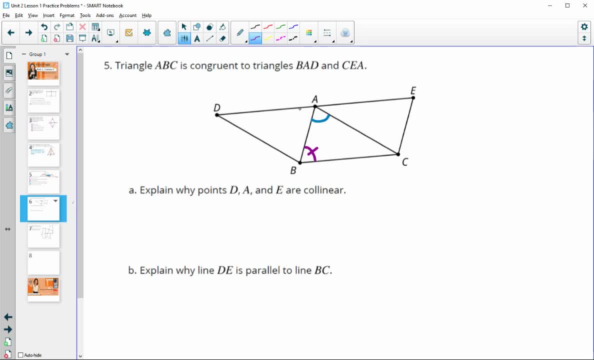 This one is actually going to be the same as this one from corresponding parts, Because it's B in this original triangle Okay, And it's A in triangle BAD. They're in the same spot, So I know those are the same. 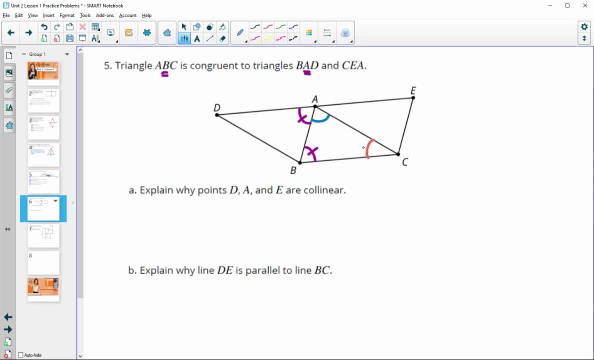 And then, if I look at this angle here, This one is the same as this one. Again, it's C in the original And it's A in this one, So they're in corresponding Spots, And then those three angles together will equal 180 degrees. 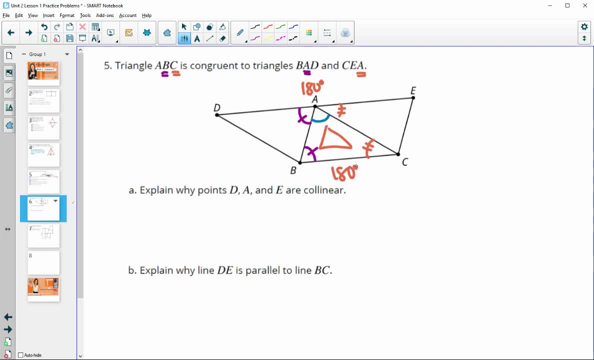 Because we know that the three angles of a triangle equal 180 degrees And it's those same three angles, So 180 degrees is a straight line. So that will create those angles being collinear And then explain why the lines are parallel. 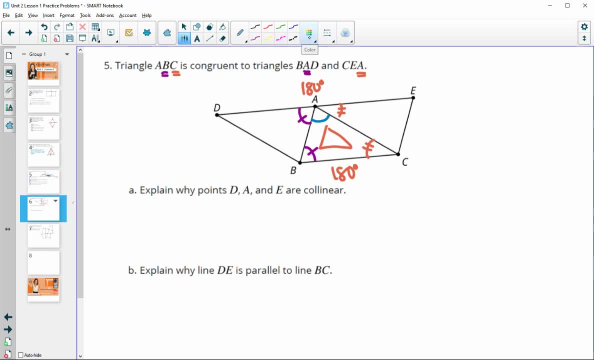 And you could explain it because of alternate interior angles. So depending on which one. But if you're looking at, you could say this angle and this angle are alternate interior. You could also do alternate interior here, But you'd have alternate interior. angles are congruent. 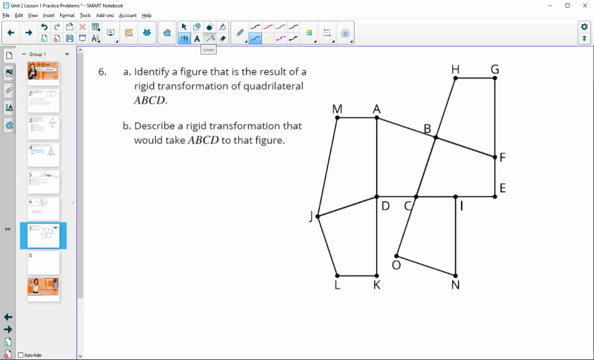 Number six Identify a figure that is the result of a rigid transformation of quadrilateral ABCD. So let's look at ABCD. It's right here Now. there's going to be multiple different answers here. You only have to pick one of them. 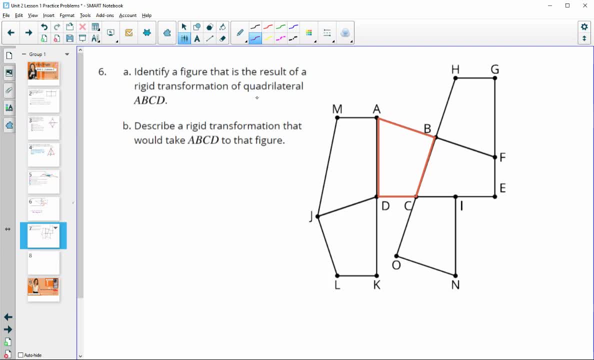 I'm just going to kind of pick a bunch of different ones here And explain for each one. So if we did this one down here- Okay, So this one here, We can see that we could translate the orange quadrilateral down. 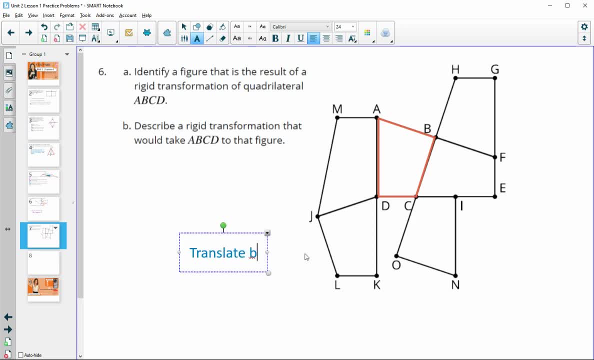 And then reflect it. So I'm going to say translate, Translate by segment AD, Then reflect across DK. So that would be again for this one. Let me color code it for you. So that would be for this one. 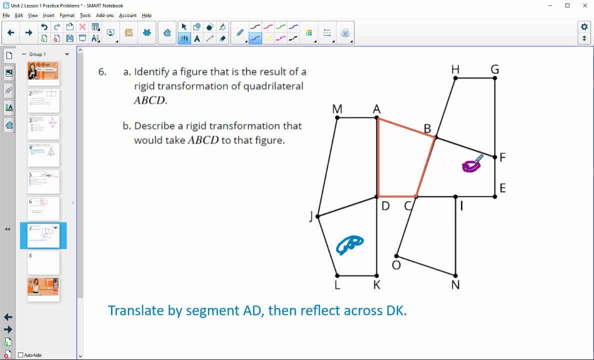 Then if we wanted to go to this one, We could say that, Let me get this colored here. So this one You just need to rotate, Okay, So rotate ABCD around. Let's rotate ABCD 180 degrees around point B. 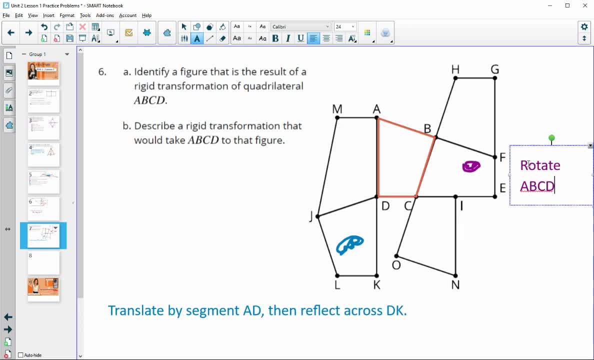 Well, and not even 180 degrees. Let's see: Rotate ABCD around point B until C coincides. Okay, So we got this one, And then we rotate C with F, since we don't know the actual angle measure. But we just want to rotate C up until F. 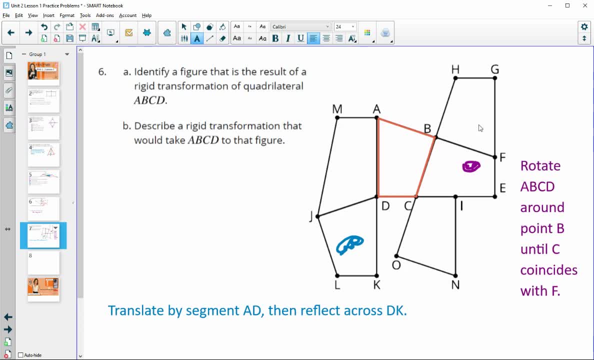 So that would be for this kind of purple one right here If we wanted to do this top one. So let me just make this one green. maybe For this one We could again rotate around, And this time it looks to be a 180 degree rotation from the straight line. 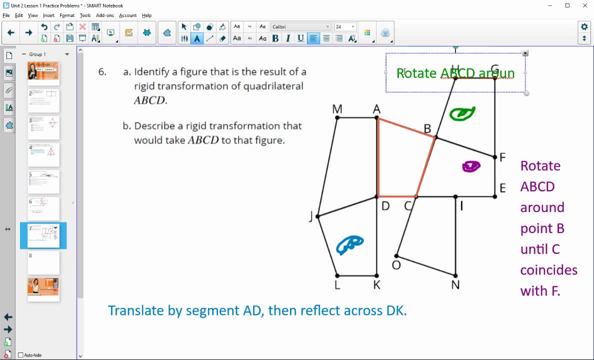 But rotate ABCD 180 degrees around A, B, C, D, around point B, And you could just say until C coincides with H, or in this case you could do a 180 degree um, 180 degrees as well if you wanted to do that instead. 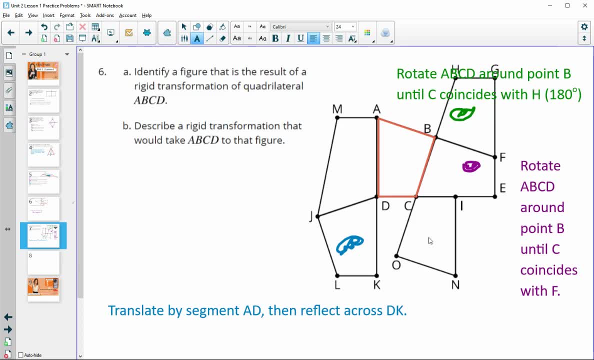 So that would be for that top one, And then this one down here also works. So let's um, do this one here, Whoops. So we'll do this one, Um and this one. you, um, we want to get um DC to land here? Okay, And then where we want to get those matched. 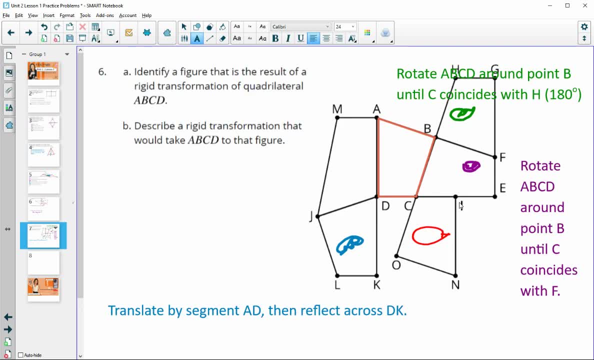 up And then this AD matches this IN. So, um, maybe we let's see what could we do here. Looks like we can just rotate it right. So just rotate, because on D you'll land here, A you'll land on N. So rotate A, B, C, D. 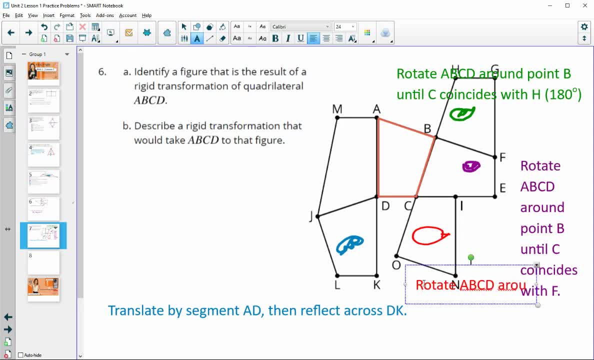